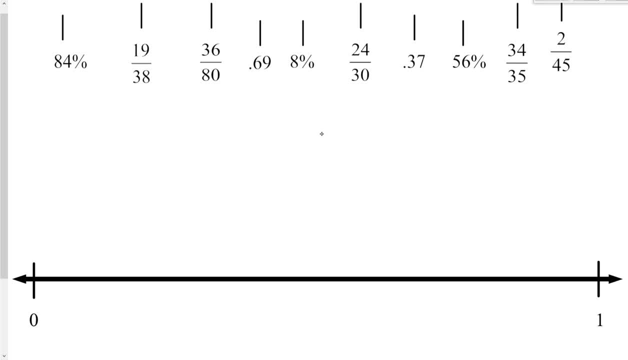 Let's take a look at another number line. This time it's not going to include just fractions and decimals, but now we're going to include percents, which is really just another form of a fraction or a decimal. Now I'm going to use the same steps that I did before, So my first step is to be: 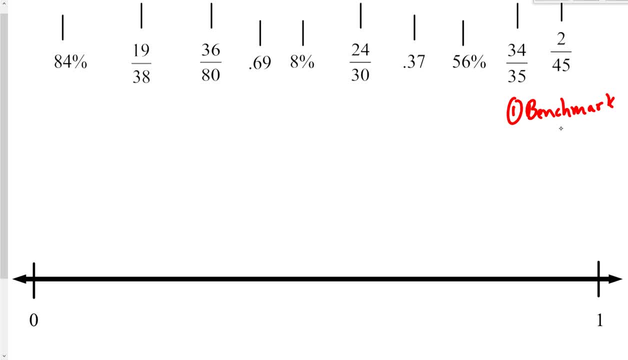 thinking of my benchmarks. Now, my benchmarks are going to be the one half, the one fourth and the three fourths, So I start by finding one half. Now, since I'm also dealing in decimals and percents, I'm going to let myself remind myself that that's the same as 0.5 or five tenths, and 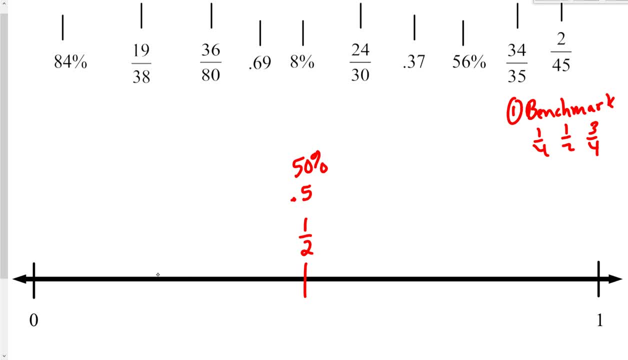 50 percent. Then I'm going to find one fourth which is 0.25 or 25 percent, and then three fourths which is 0.75 or 75 percent. Now the second step. I'm going to simplify where I can because I might. 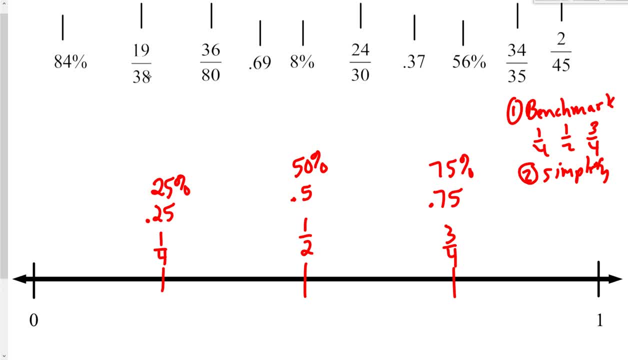 be able to make some things easier for myself, Like, for instance, 19 thirty-eighths- that's one half. That's really good to know. 36 eightieths- I know I can simplify by four, So that's going to. 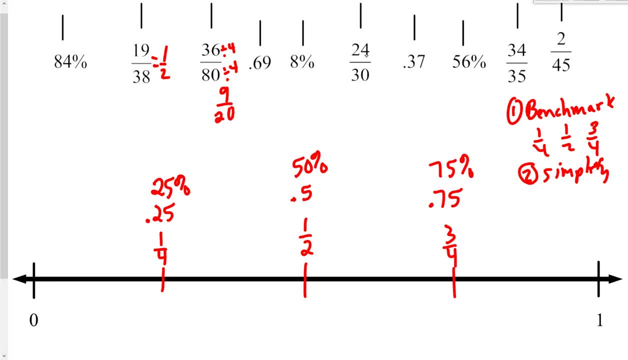 be nine, twentieths, 24, thirtieths- I can simplify that by six, So four, fifths, And that's all that can be simplified. Now, the next thing I want to do is I want to start thinking about close to zero, one half or one. 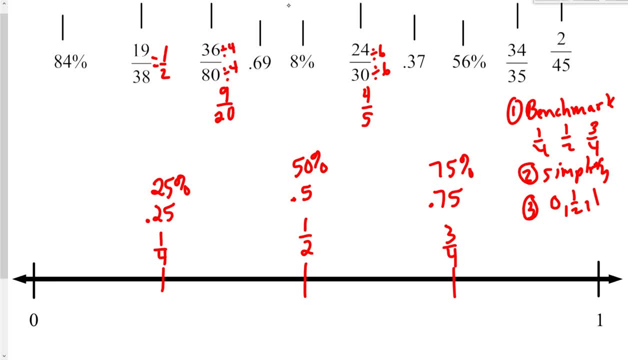 whole. So I'm going to go through and do that. 84 percent, that's up near one whole. One half, well, that's exactly one half. Nine twentieths, That's about one half, but it's actually going to be a little less, Because ten twentieths would be one half. 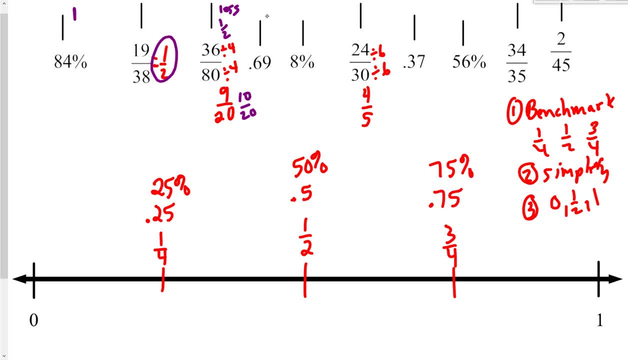 69 hundredths we're getting close really to. I'm going to actually put three fourths for that one, because I know that that's where it's near. 8 percent is near zero. Four fifths is near one whole. But I'm starting to think I recognize something about four fifths. 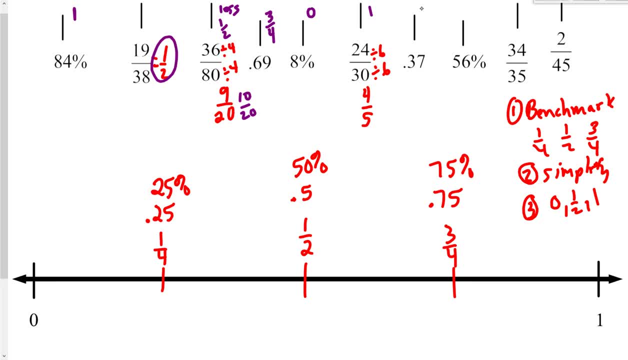 I'll come back to that. 37 hundredths, that's between one fourth and one half- 56 percent is about one half a little bit bigger- 34 thirty-fifths, very close to one whole, And then two forty-fifths down near zero. So now that I have my zero- one half and one whole- I can start. 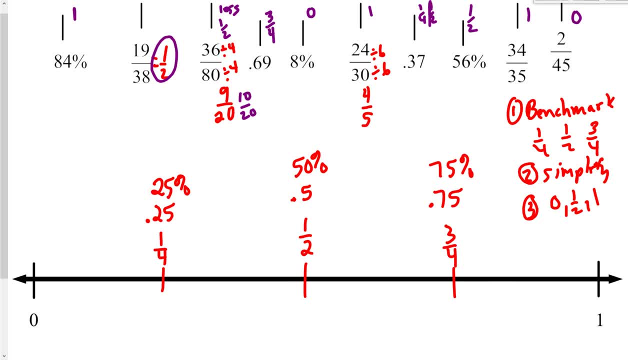 moving some of my fractions around. Last thing I want to point out, though, is that oftentimes I will be thinking in percent, Because if I know the percent of a fraction or a decimal, then I can more easily start to place them on my number line. 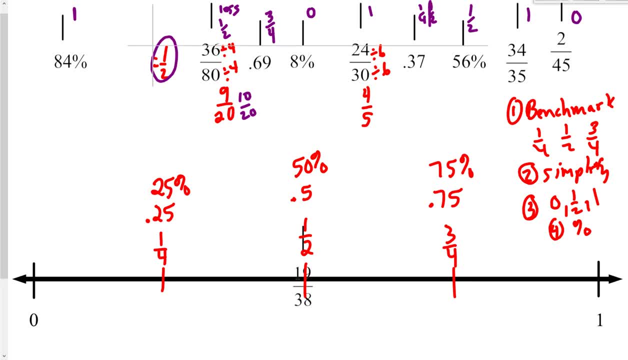 So I'm going to grab some of the first obvious ones, like 19: thirty-eighths is one half, So I'm just going to put that right on there, Okay, and then I look for some other ones that might be standing. 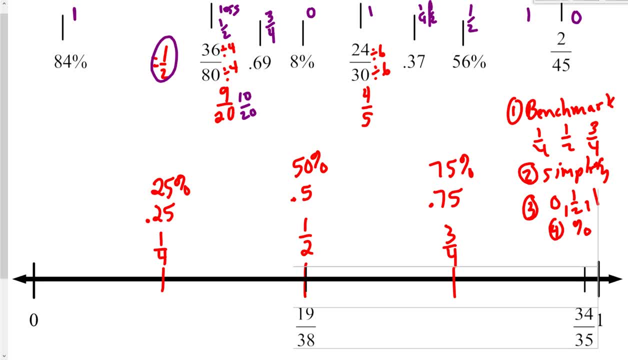 Anyhow, 34 thirty-fifths, that's close to one whole, So I'm going to put that up there. My two forty-fifths: well, that's pretty small, So I'm going to put that down near zero. 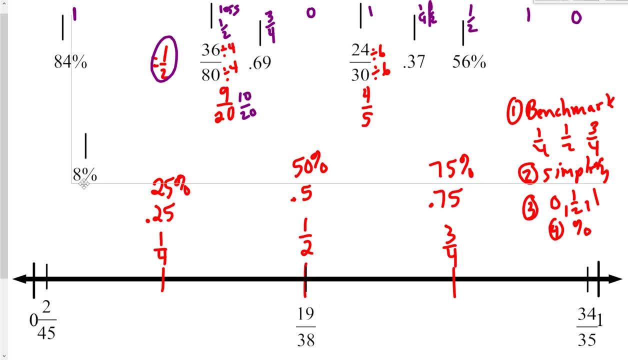 But then I remembered I had eight percent And I have to start thinking about eight percent and two forty-fifths. Well, this is where it's helpful when I'm thinking about what I know about percent. Well, I know that eight percent means it's eight hundredths. Now, I can't make forty-fifths to hundreds, but I can. 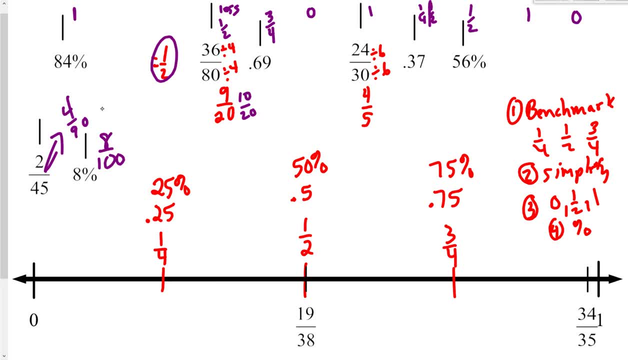 make this 4- 90th- and I realize that there's even. if I were to go to hundredths, it's probably not even going to be five, so let's call it 500 too. so we'll say it's about 500, which means that my 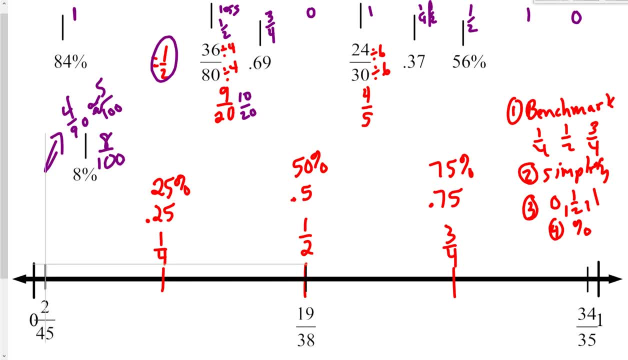 four to 45th is definitely less than my eight percent. okay, so those are my two smallest ones. now I'm going to start peeking around for some more things. I have another one, close to one half. since it's a percent, I know it's a bit more than a half. 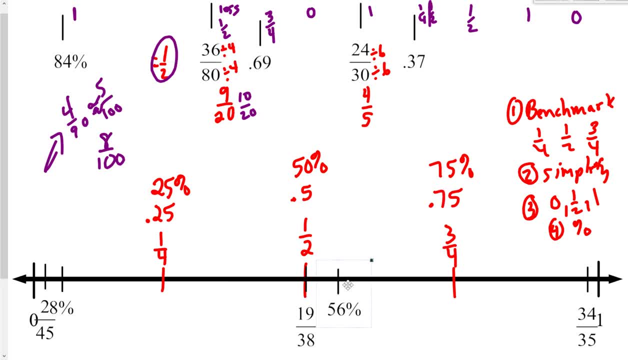 because it's 56 percent. I knew I had another one. oh, here it was. this one here is close to one half. it's a little bit less than a half, so I'm going to bring that down here, place that one less than one half. then I'm going to start grabbing some of the others 69 hundredths. well, now the nice thing. 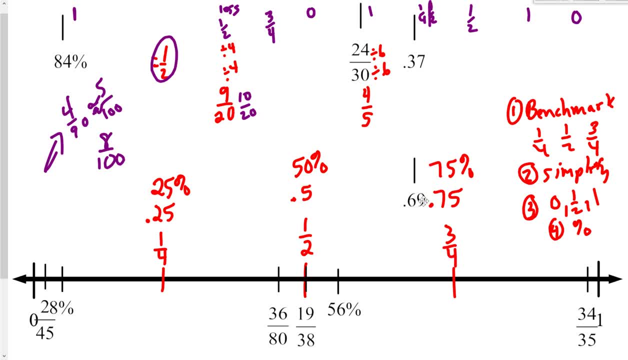 this is why I use the decimals in my benchmarks. it's a little bit less than 75 hundredths, so I can place it right about there. here's my 37 hundredths. well, that's going to be a bit more than 25 hundredths. in fact, it's pretty much right in the middle of 25 and 50, so I'm 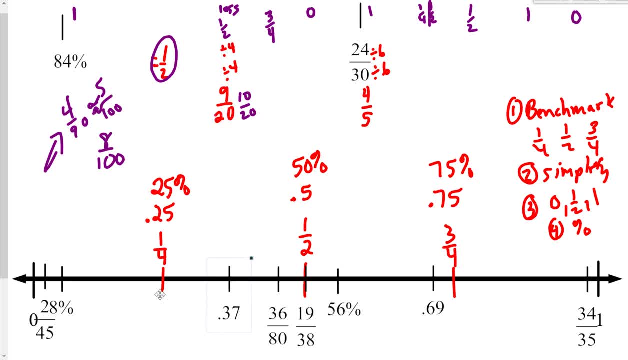 going to put that pretty much right in the middle there of one fourth and one half, using my benchmarks to help me. so now I have two left, I have 84 percent and I have 24- 30. now both of those I know are near one hole. now let me just erase some of these things around kind of getting in. 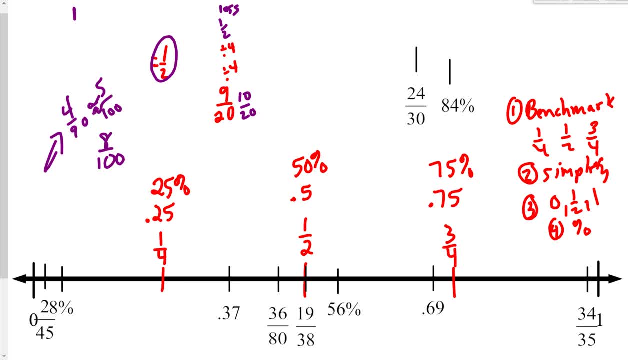 the way. now I know, as a reminder, that this was four fifths. now, if I want to be able to compare that to a percent, I want that to be out of. Well, I know 5 times 20 is 100, so I'm going to do 4 times 20 and get 80. 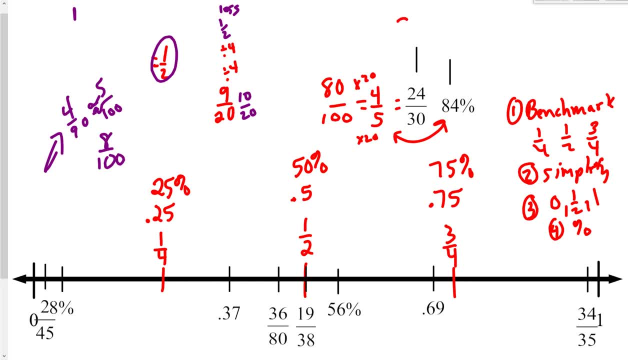 So that means that 24- 30ths is 80%. So 24- 30ths is a little bit more than 3- 4ths, because that's 75%, And then 84% is going to be a little bit more than that. 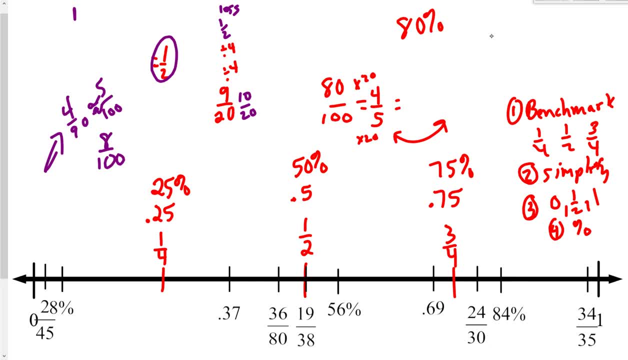 And that is how I would place those fractions on my number line: N decimals, N percents. Again, those are my steps.